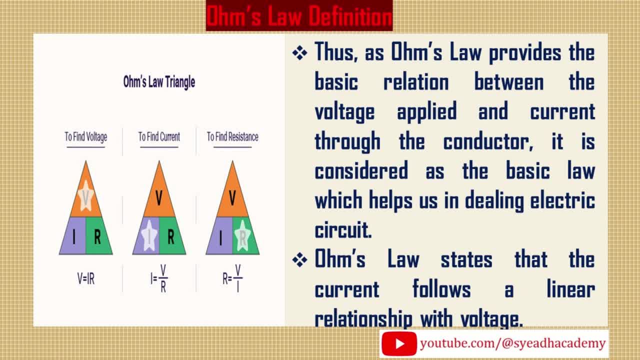 the conductor. it is considered as the basic law which helps us in dealing electric circuit. Ohm's law states that the current follows a linear relationship with voltage. Ohm's law explanation. Ohm's law is one of the fundamental laws of electrostatics, which 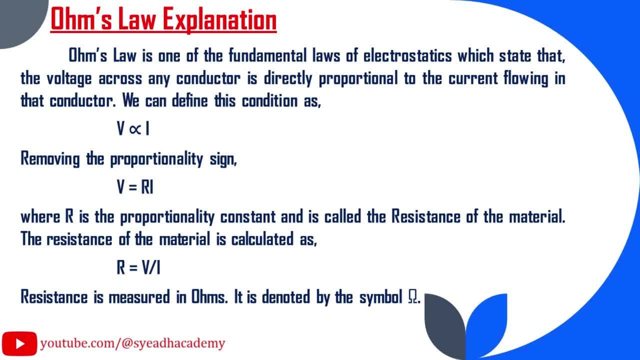 states that the current flows through the conductor and the resistance of the current flows through the conductor. Thus, as Ohm's law states that the voltage across any conductor is directly proportional to the current flowing in that conductor, We can define this condition as: V is proportional to I, removing the proportionality sign V, equals R- I, where R is the proportionality. 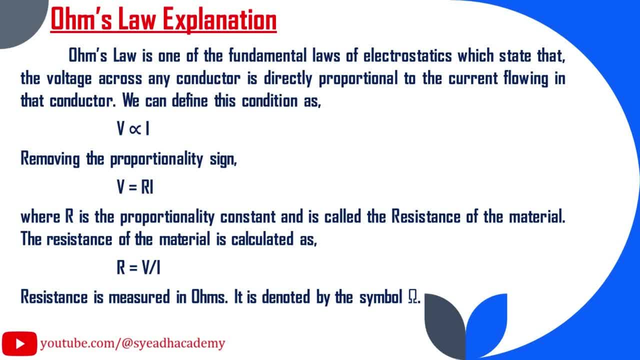 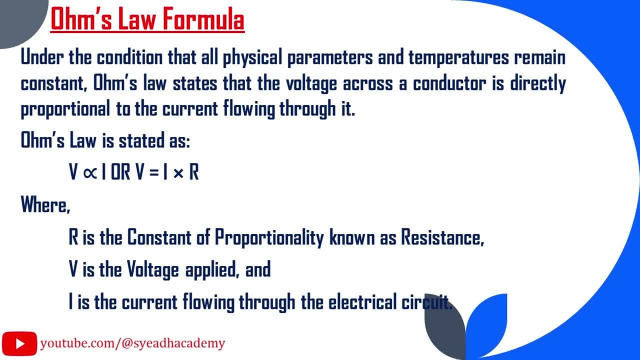 constant and is called the resistance of the material. The resistance of the material is calculated as R equals V divided by I. resistance is measured in ohms. It is denoted by the symbol omega Ohm's law formula. under the condition that all physical parameters and temperatures remain, 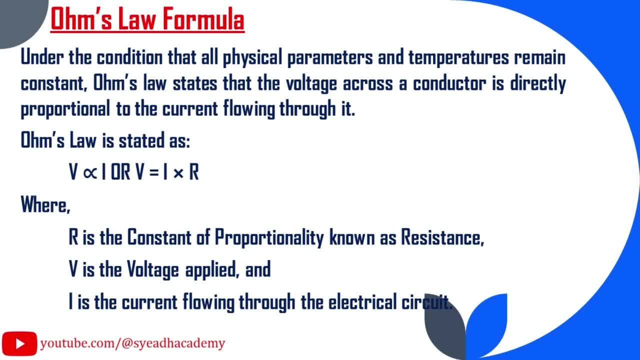 constant. Ohm's law states that the voltage across a conductor is directly proportional to the current flowing through it. Ohm's law is stated as: V is proportional to I or V equals I into R, Where R is the constant of proportionality, known as resistance, V is the voltage applied. 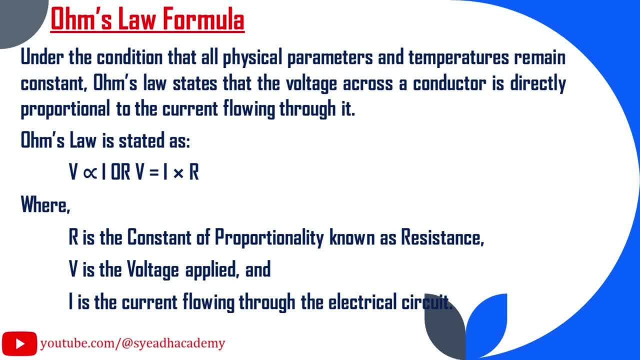 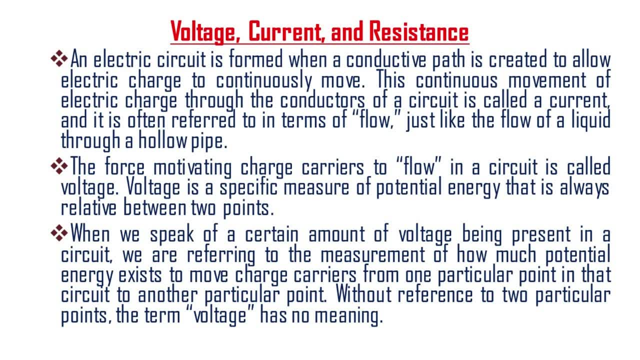 and I is the current flowing through the electrical circuit: Voltage, current and resistance. an electric circuit is formed when a conductive path is created to allow electric charge to continuously move. This continuous movement of electric charge through the conductors of a circuit is called a current and it is often referred to in terms of 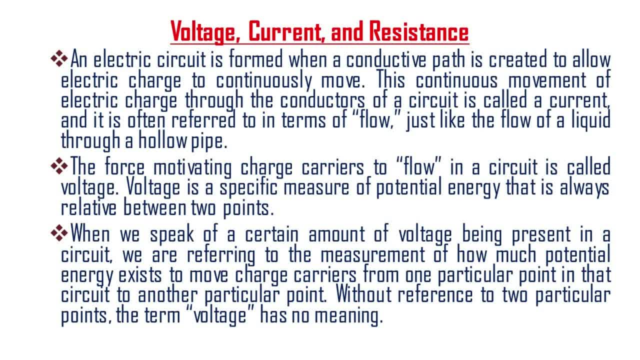 flow, just like the flow of a liquid through a hollow pipe. The force motivating charge carriers to flow in a circuit is called voltage. Voltage is a specific measure of potential energy that is always relative between two parts of the circuit. Voltage is a specific measure of potential energy. 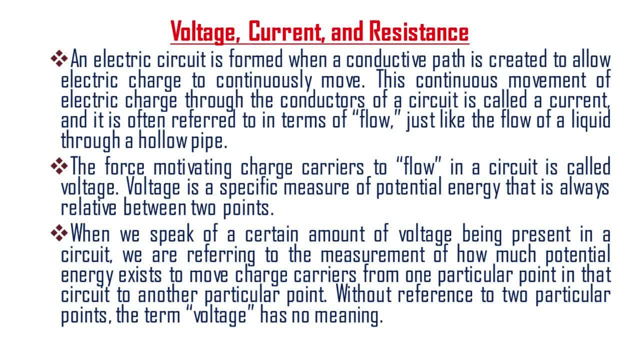 that is always relative between two parts of the circuit. When we speak of a certain amount of voltage being present in a circuit, we are referring to the measurement of how much potential energy exists to move charge carriers from one particular point in that circuit to another particular point. Without reference to two particular points, the term voltage has no meaning.